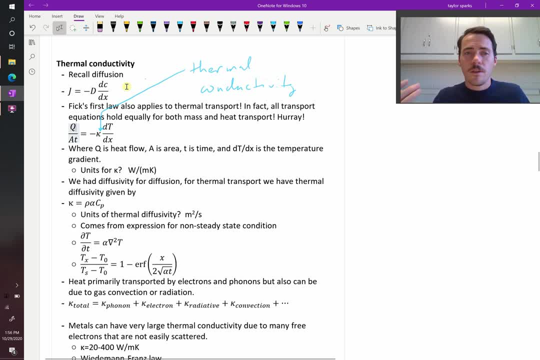 With diffusion. here we call it Fourier's law, but it's the same thing, okay. So again, I've written out here: q divided by a times t, because we had to make it a flux. q is just energy. So if we want, 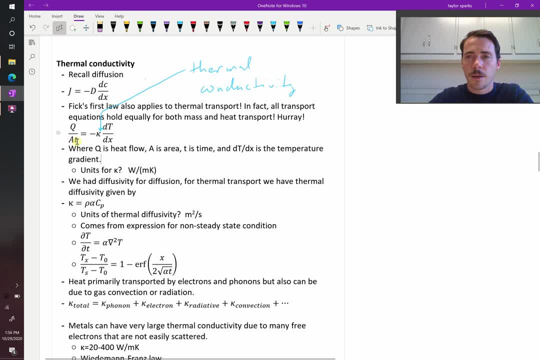 the flux of energy. then we have to do q per area per time. right is equal to negative. kappa our thermal conductivity times dt dx, where that's the temperature gradient. okay, So what would the units be? The units of thermal conductivity are watts per meter kelvin. okay, Where? remember a? 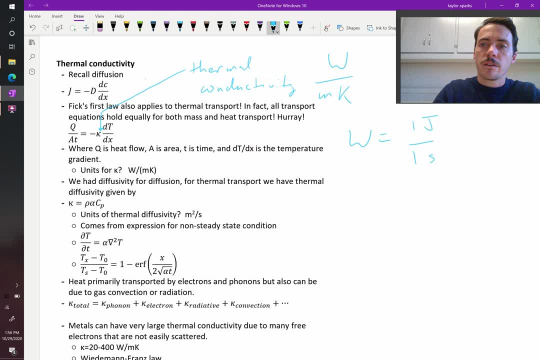 watt per meter kelvin is the temperature gradient. So what would the units be? The units of thermal conductivity is equal to one joule per second right. So joule is going to be our measurement of energy. How many joules right? Okay, Now there's another important term, The one difference between: 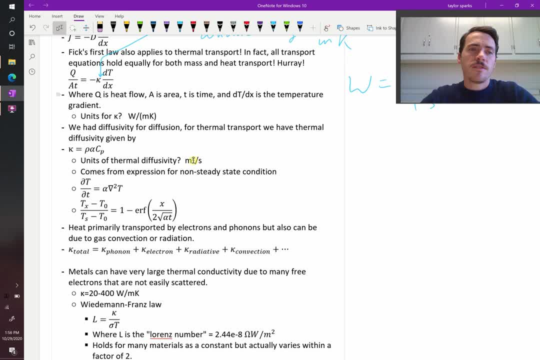 thermal mass transport and heat transport. is that, when it came to the second, non-steady state diffusion right, where we figured out how things change, how, where we calculated the composition as a function of position, when time is changing, when the rate is changing? 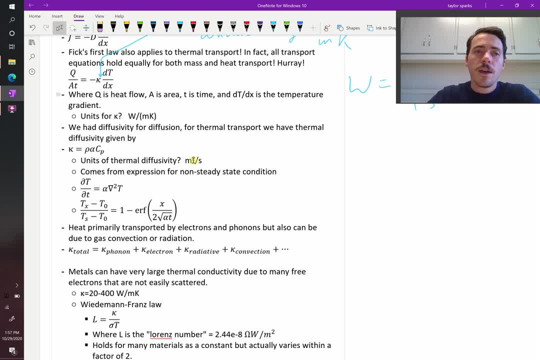 we used diffusion there and we used it in Fick's first law. With thermal transport we have to use a different parameter. We have to use thermal diffusivity. So what is that All right? Well, thermal conductivity is right here. Kappa is equal to rho times, alpha times, cp. Rho is our density. 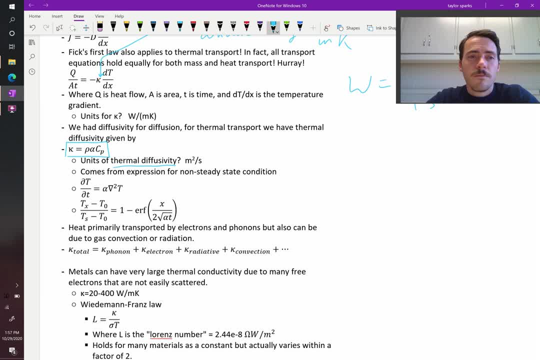 right? Alpha is our thermal diffusivity and cp is our heat capacity at constant pressure, right? So let's just do a quick unit analysis here, right? Thermal conductivity had watts per meter per Kelvin, right? So this is going to be equal to density, So that's just do. kilograms per meter cubed, just to put these all. 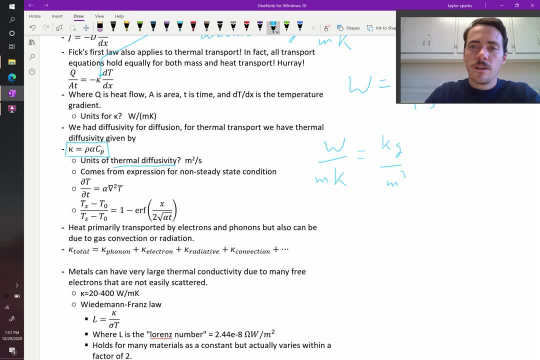 in SI units. right Multiplied by our thermal diffusivity, right Multiplied by heat capacity, We know that that's joules per kilogram, per delta T, right? Some difference in temperature like Kelvin. So let's just write that as Kelvin. So what must be the units of this? 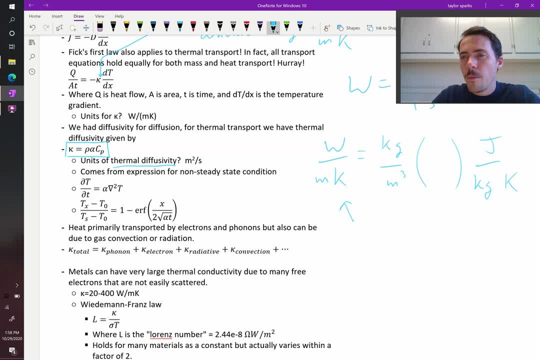 one right here in order to end up with this over there. Well, remember that a watt is equal to a joule per second, So we can rewrite this as joules per second, meter cubed, right. So in order to get meters alone down here, we need to have a meter squared up there, And then our kilograms are. 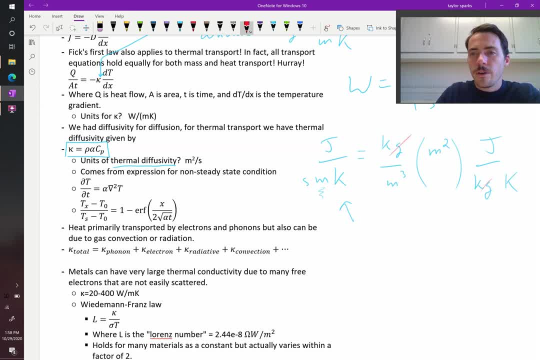 going to cancel, right. So what we need now is seconds. So this needs to be meters squared per second. This has the exact same units as the diffusion coefficient. Remember when it was mass transport, the diffusion coefficient also had area per time. It was typically centimeter squared. 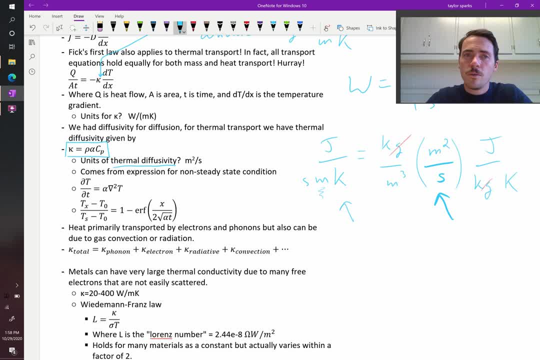 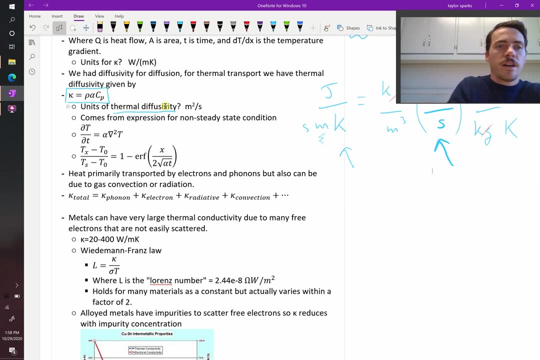 per second. but you know, meter squared per second, it has the exact same units as mass transport. But now this is the thermal diffusivity, not the diffusion coefficient. okay, So that alpha value, that's what we're going to use with Fick's second law for thermal transport. Fick's second law. 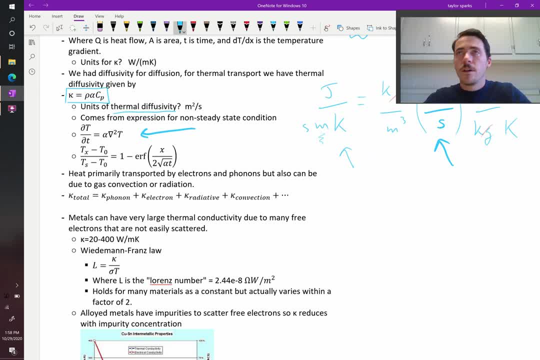 again. remember it came from the fact that our rate of temperature, our flux of heat, is changing with time. It's not constant. So now you have to take into account that the flux of heat is changing out time. So d temperature, d time has to be equal to this partial differential equation where it's 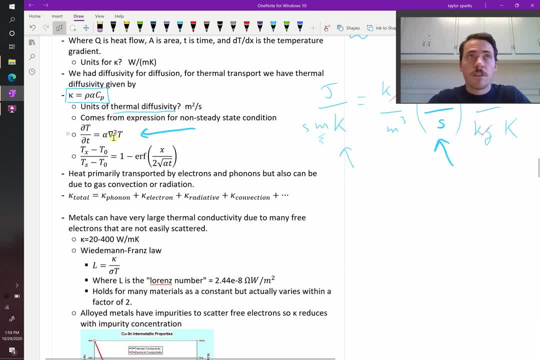 thermal diffusivity times, the gradient second derivative right, The gradient in temperature, respective position. So nasty equation. We don't have to solve it on this class. Instead, we're going to use a solution, and it's the exact same one that we saw for mass transport. How cool is. 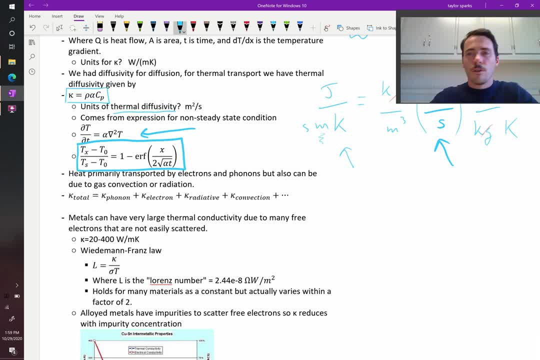 that, Whether you're describing heat or mass moving through material, it's the same equations. Before it was the composition at point x, Now it's the temperature at point x Minus the temperature that's deep within your material right. So again, if you have this, 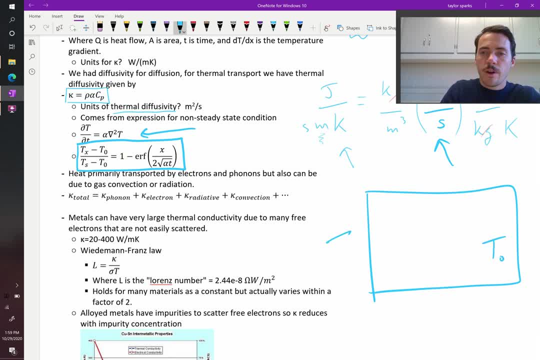 scenario: somewhere far within your material it's T0. But then, right here at the surface, you heat it up. So right at the surface, now you've got it hot. okay, So Tx minus T0 divided by Ts minus T0, where Ts is the temperature right at the surface- is going to be equal to 1 minus the. 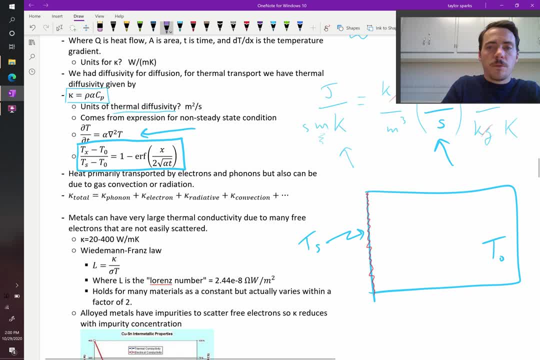 error function of x, your position. x is going to be your position going this way. So that's x, Right? there would be x equals 0.. Over here would be x equals infinity, right, Infinitely. in your material, you have a temperature of T equals 0. And then, divided by 2 times the square root of 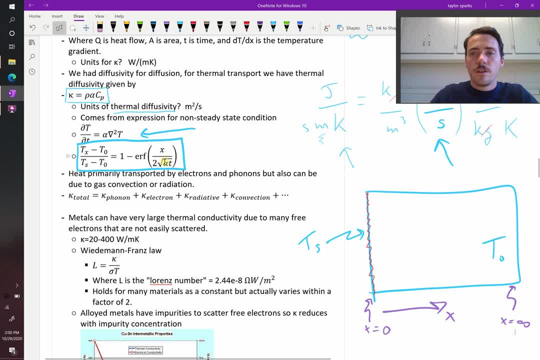 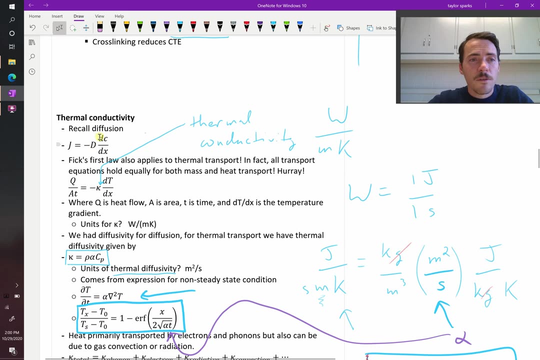 alpha T, where alpha is your thermal diffusivity, right Thermal diffusivity. So that's the key difference is that you plug that in for alpha right there. If it was mass transport, then the diffusion coefficient, you used it both in Fick's first law and Fick's second law For mass. 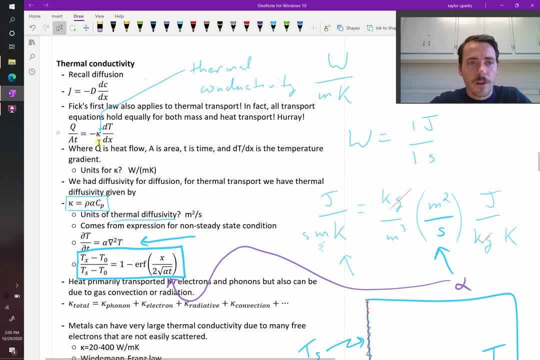 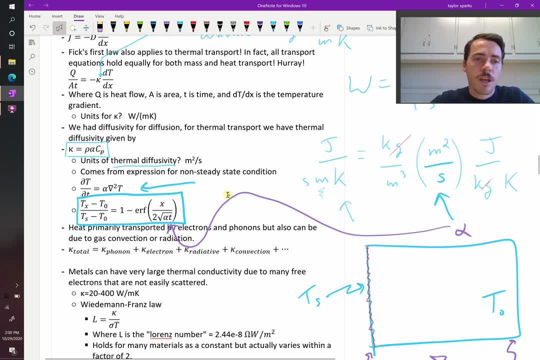 transport. the only difference is that for Fick's first law you use thermal conductivity, kappa right here, But for Fick's second law you use alpha there. Otherwise they're the exact same. okay, So let's talk about thermal conductivity for a minute. What makes a material a good? 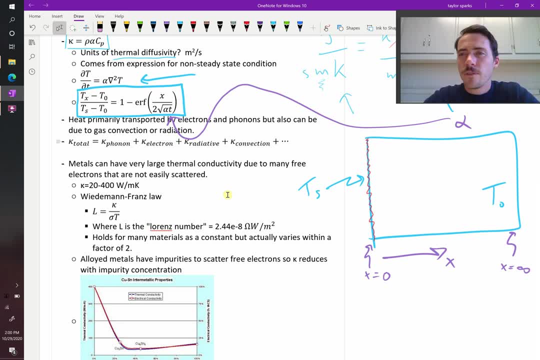 conductor of heat versus a poor conductor of heat? To answer that, we first have to think about how heat gets carried in a material. What actually carries heat in a material? Well, the total conductivity is going to be made up from contributions from lots of things, right As. 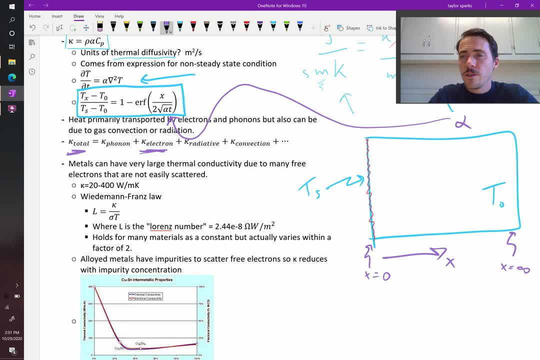 electrons move through your material, they can carry heat because they have a kinetic energy with them. You have phonons, right, Those lattice vibrations. as they move through your material, they can carry heat. You can have radiative transport of heat. That's when, like the sun, 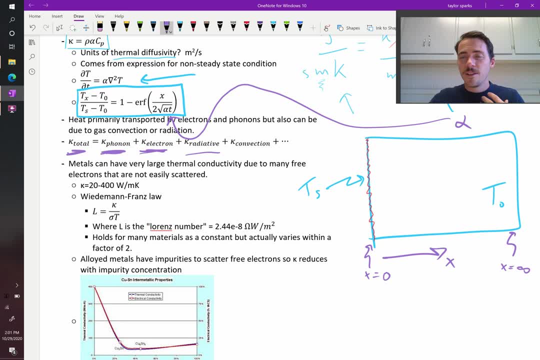 it's a giant radiated thing. We're not touching it, so it's not like electrons or phonons are traveling to us. but there are photons, right? Photons, that light coming off, that's radiative, right, That's electric. 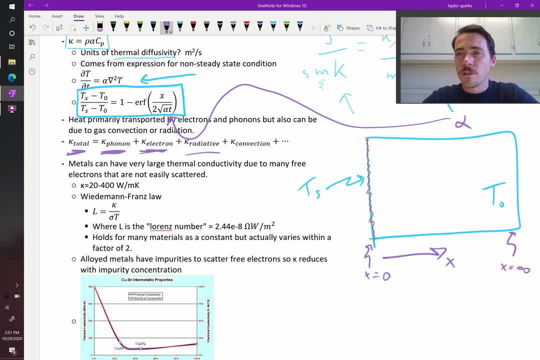 Electromagnetic radiation coming off of something. if you heat up your stove and you see it start to glow red, you're seeing that radiative heat and you can put your hand near it and you can still feel it. That's radiative transport. And then there's convection, which is basically forced. 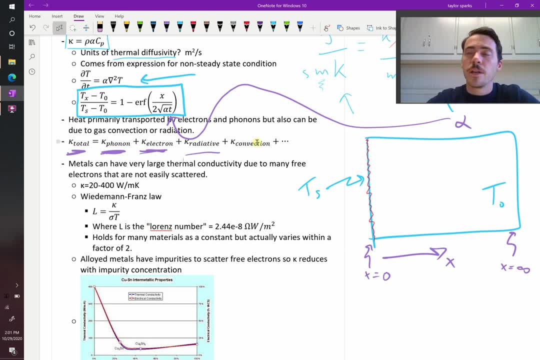 air when air gases or liquids are being pushed at an object. This is why we blow on our soup. If you've got a hot bowl of soup, you blow on it because you convectively have your breath touch the soup and then carry that heat away with the moving breath. So think of it as like fluid flow. 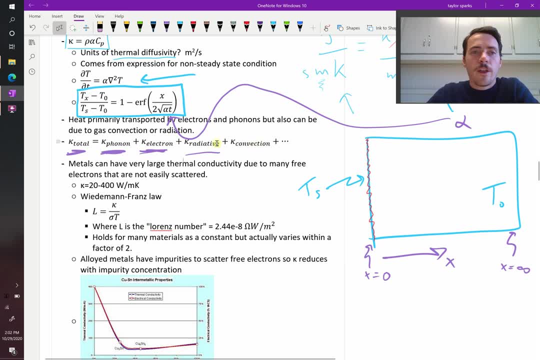 it's a gas or a liquid fluid, okay, All right. so now that we know that those are the things that can carry heat, that can contribute to thermal conductivity, now we can dive into whether things should have a high or a low thermal conductivity. Let's start with metals. Metals should have a 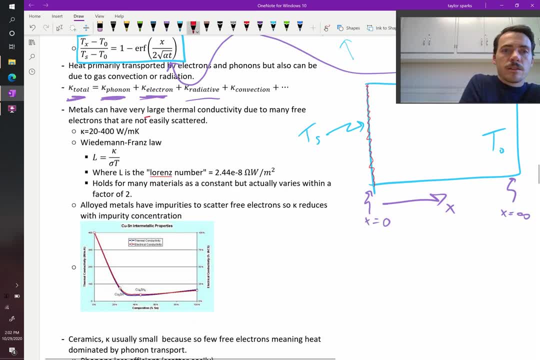 really high thermal conductivity. Why is that They should have a large thermal conductivity? because they have three electrons. Metals are defined by having lots of electrons available to carry electrical current right. They can also carry heat. That's why if you go cooking marshmallows- 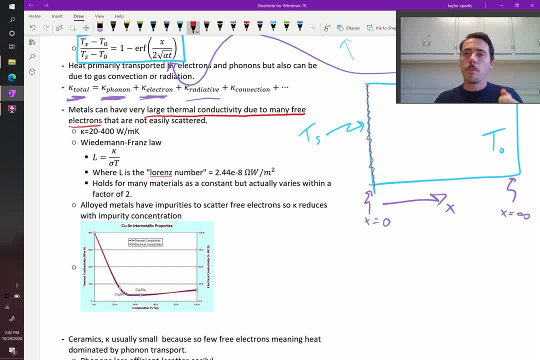 and you have a stick with a marshmallow on it, your hand's probably not going to get warm. But if you've got a coat hanger with a marshmallow on it, there's a very good chance you're going to burn your hand. because that coat hanger is metal. it's got electrons. it's going to conduct heat really. 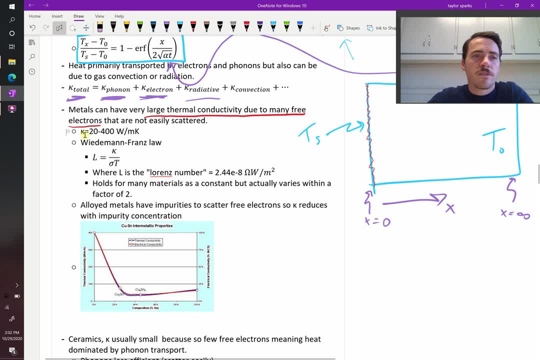 well and you might actually burn your hand okay. So typical values are something like 20 to 400 watts per meter kelvin. for metals. We have something called the Wiedemann-Franz law which says that there's a constant the Lorentz number right given right here 2.44 e to the. 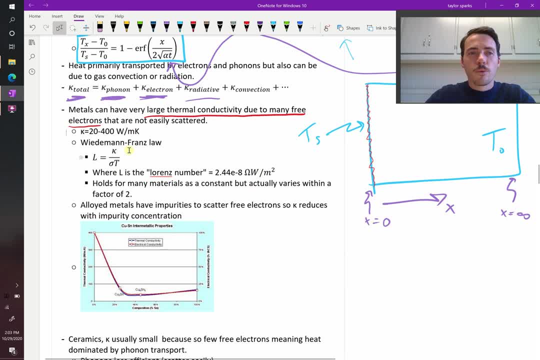 negative eight ohm watts per meter squared and that's equal to the ratio of thermal conductivity to electrical conductivity times temperature. So we're going to talk about that more when we get to electrical conductivity in a couple of chapters. But you know this is not a law, in that it's. 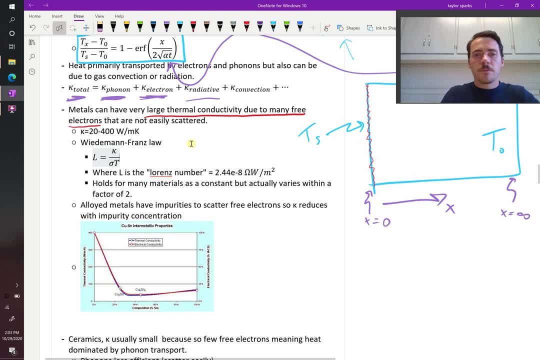 unviable. It holds for many materials, but there are exceptions. For most materials it holds within a factor of two. So you can find things that kind of break it. It's rare to find something that really breaks it, Something, for example, that would be an excellent conductor of electricity. 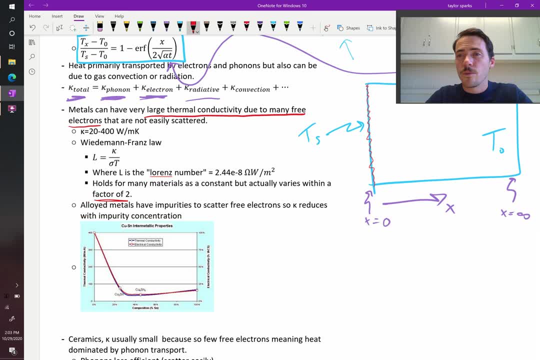 but a rotten thermal conductor. We actually want those for things called thermal electrics, which we'll talk about in a few chapters. We'd love something that conducts electricity- great- but will not conduct heat. But typically, if you get one, you get the other. If 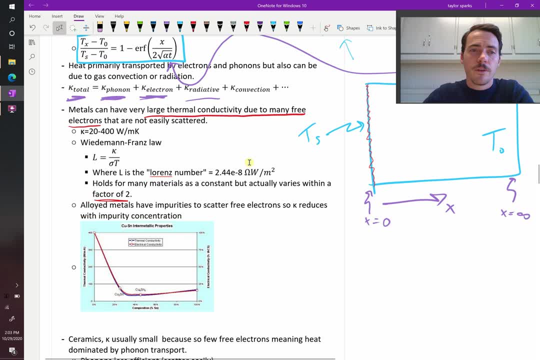 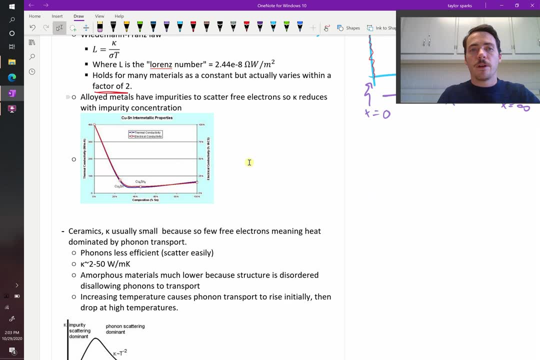 it's a great conductor of heat. it also conducts electricity, and it's hard to decouple those two things right. That said, you can reduce the thermal conductivity of metals. One way to do that is to alloy your metal. As you form an alloy, think about what you're doing, right, You start. 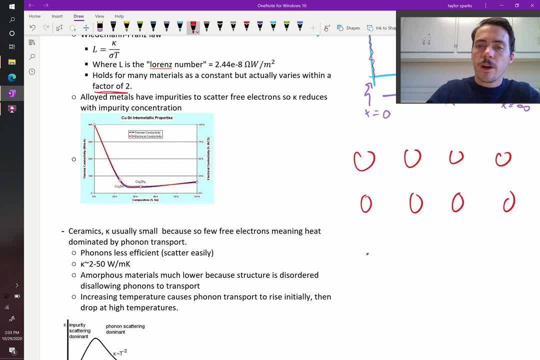 out with a nice regular lattice of some sort of metal right. And when you alloy it, let's say we start to substitute out some of these atoms with others, We start to substitute out some of these atoms with others. So now this one's a different atom, this one's a different atom. Well, when you 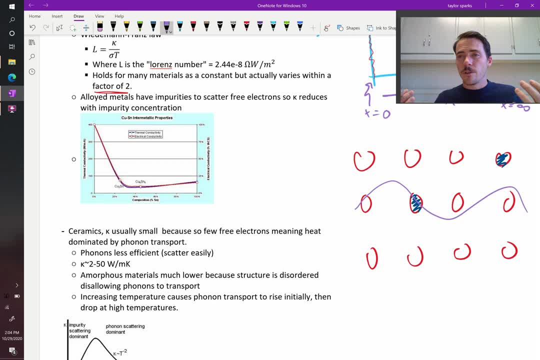 had your wave of atoms, let's say you had like a wave, a phonon, traveling through material. it now could get scattered off of this one. They can act as scattering sites for your electrons or your phonons, both of which carry heat, And if you scatter them, then they don't carry heat as well. 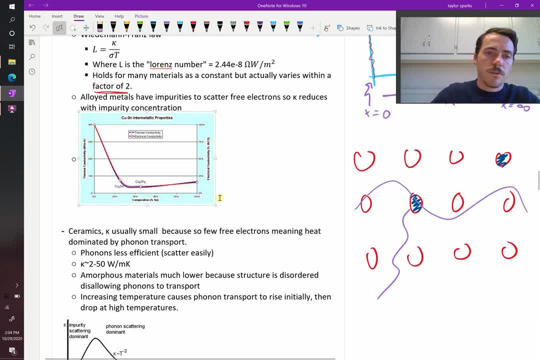 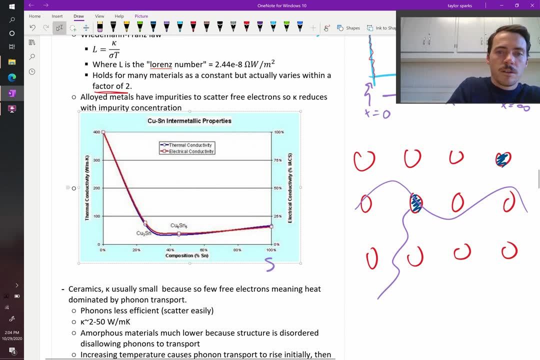 So that's typically what you see here. Take, for example, in this plot. Here they're showing you in this plot they're plotting thermal conductivity as a function of composition, So as they go from pure copper over here to pure tin. so this would be tin and this would be copper. You've got copper. 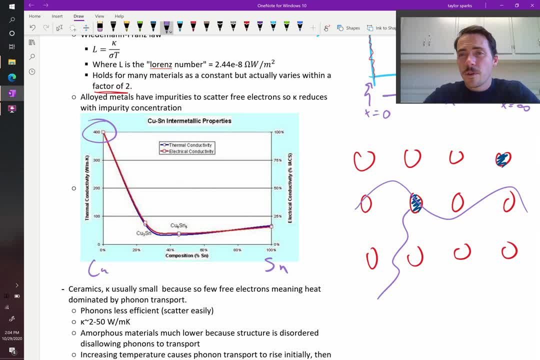 which has 400 watts per meter Kelvin. It's one of the best thermal conducting metals we have. It's a really good thermal conductor. But as you introduce tin, this thing just plummets. By the time you're at 20% tin it's cleared down. you know. it's dropped by a factor of four or more right And 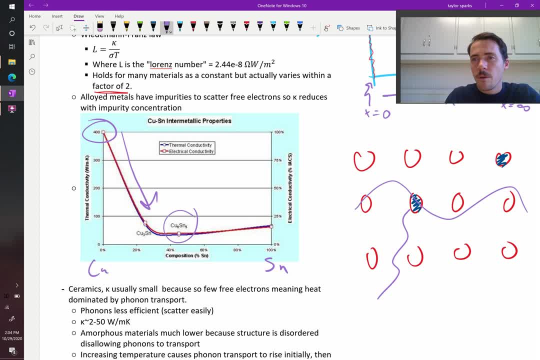 then when you're at 50-50, that should be about your lowest right, Because that's the most disorder that an alloy can get is when you have equal parts of the two elements And as you come up it rises again just a little bit to whatever the value it was for pure tin, which 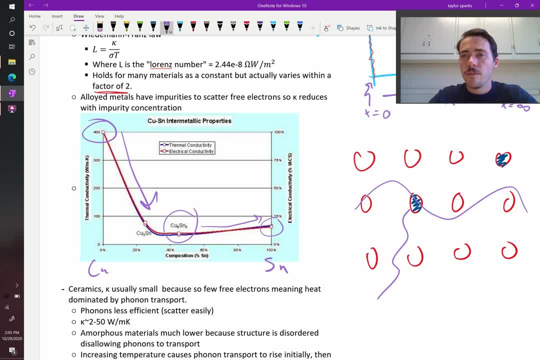 doesn't have to be the same as copper, because copper, we know, is certainly more conductive than tin, But there could be other factors like how phonons interact in the material as well. okay, All right, so that's metals, and thermal conductivity typically pretty high. What about? 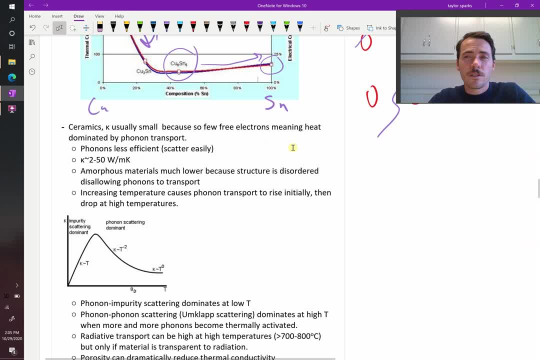 ceramics. Well, ceramics it's usually small because there are very few free electrons, right? So that's remember, if our total thermal conductivity, kappa right, is equal to kappa electronic, plus kappa from phonons, plus kappa from radiation and so forth, right, If you just 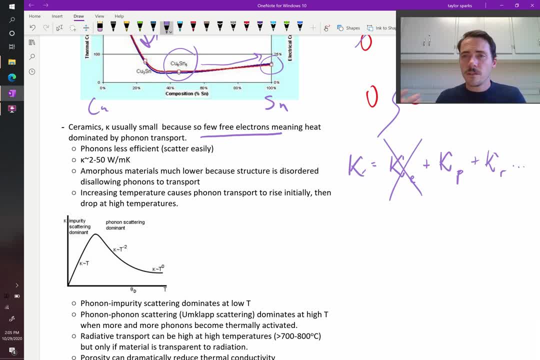 get rid of one category because there's no free electrons. you'd expect it to have a lower thermal conductivity And sure enough, that's what we get here. It's typically lower and it's dominated by phonon transport. right, This phonon term is the really important one. So lattice, vibrations and 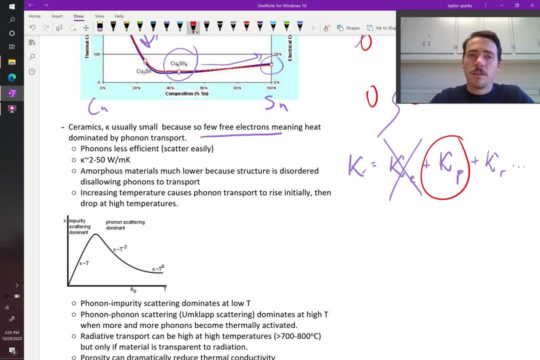 ceramics are the key ones for them to be good conductors or bad conductors, right? So if you take a material where they can just be conductors, right? So if you take a material where they can be scattered, then it's going to be a less efficient conductor, right? That said, typical. 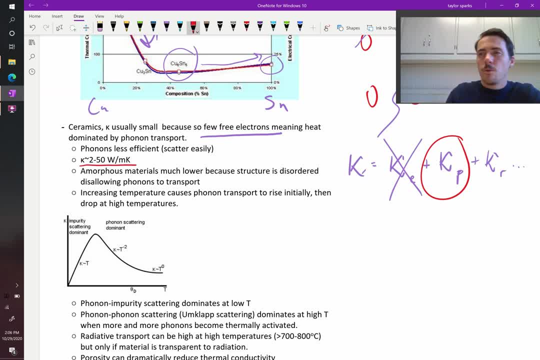 values for thermal conductivity and ceramics is something like 2 to 50 watts per meter Kelvin. A lot of the oxides that are around us- you know that make up dirt all around us- are going to be pretty low: 2 to 10, probably even less right. It's rare to find ceramics that have a lot higher. 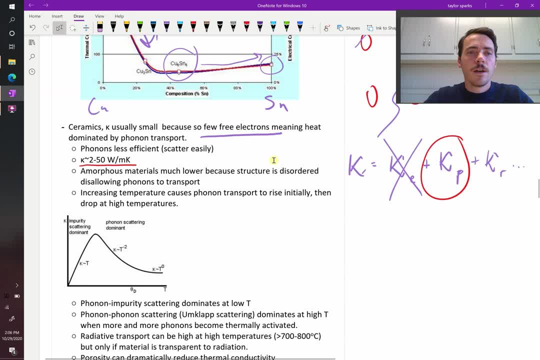 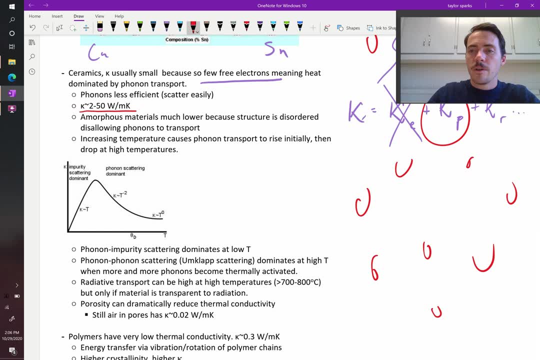 values, but they do exist. We'll give you an example in a minute. The more amorphous ceramics, right? Remember, an amorphous ceramic doesn't have a regular structure, It's just this random arrangement. Think about how a wave is going to travel through that material, right? 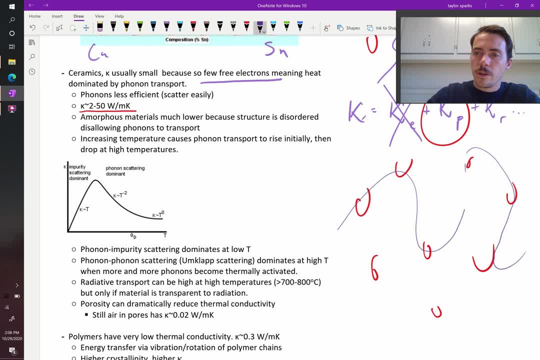 How much harder is it for it to form a wave of atoms when they're all over the place? right, It's much harder. So these are really low thermal conductivity materials, because they don't have good phonon. They don't have ways for the phonons to travel through them efficiently. Instead, 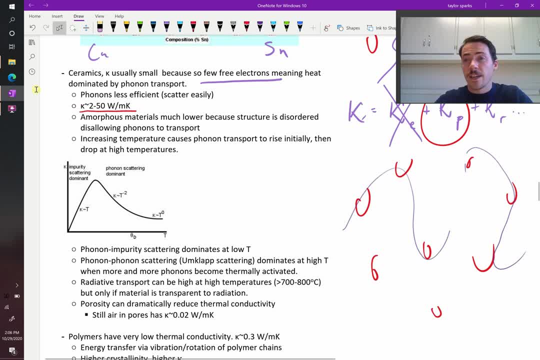 they get scattered off of the disordered structure. So amorphous materials like glass, like what we make our windows out of in our homes. they are great in that they're transparent and great in that they don't conduct heat very well, which is good because we want to be able to see. 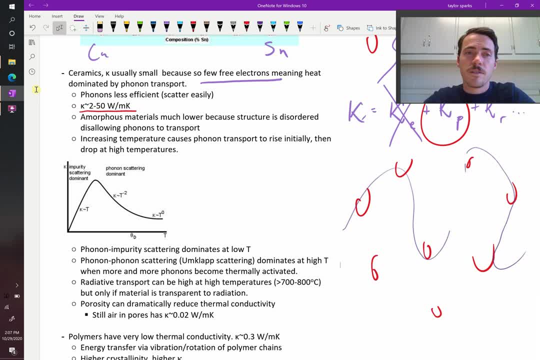 outside, but we don't want to lose a lot of heat through our windows, So it's nice that amorphous materials like glass are also low thermal conductivity materials due to their disordered structure. right Now, thermal conductivity has a typical temperature dependence, right. 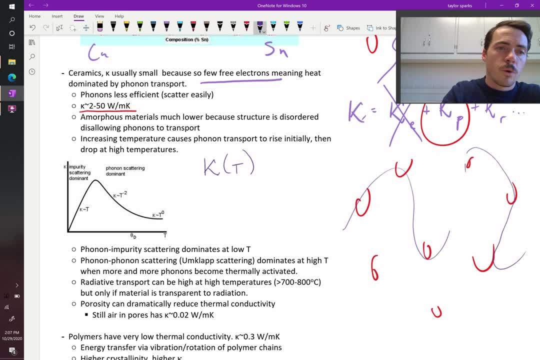 Thermal conductivity has a typical temperature independence, where it rises at first. The reason it rises at first is because as you heat a material up, we know from heat capacity, right, What do we know If we go back up to our heat capacity as you heat it up? its heat capacity rises because you're 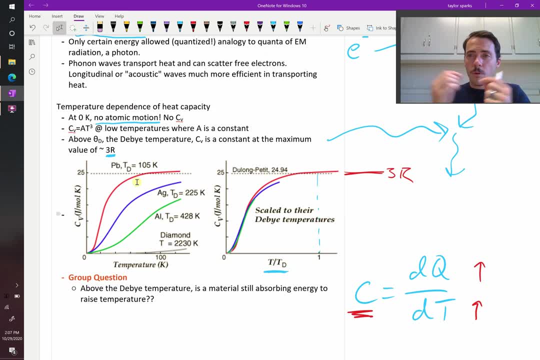 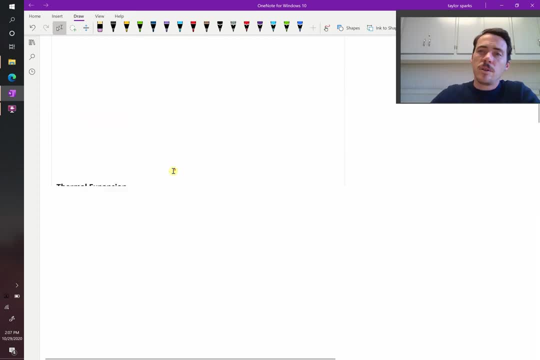 activating phonon modes, You're basically allowing things to vibrate more and more up until a point when they reach 3R, and then they're not vibrating at a greater rate, They're just maxed out at how they vibrate. So as you heat something up, you're increasing your phonon modes and those phonons. 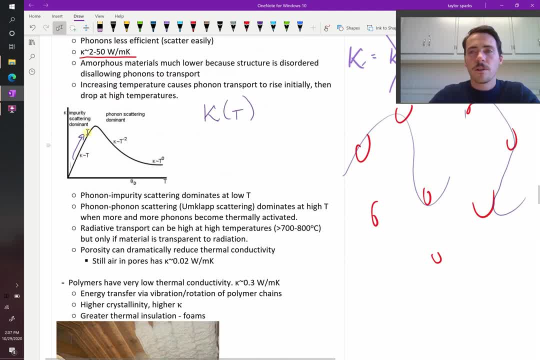 are free to carry heat. So that's why thermal conductivity rises at first, and then it reaches this peak and it starts to decline at typically like T to the negative two or T to the negative two. Why is this? Well, think of it like people in a subway station. The more people there are in a crowded 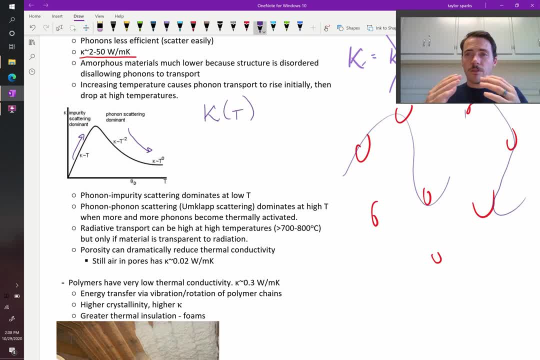 subway platform. all of a sudden, when the train shows up and the people want to get on the train, they start to move more slowly because they're bouncing into one another. right, They scatter off of one another. That's what's happening with phonons: You create so many phonons that now they 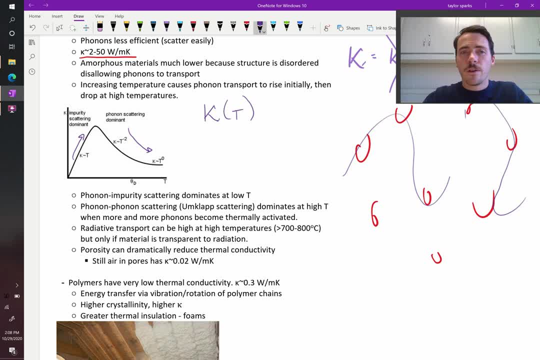 start to scatter off of one another, And so it's harder to get an overall good conduction of heat from these phonons, since they're scattered off of one another. That's why you know it's good to activate phonons in terms of increasing thermal conductivity over here, But if you get too many, 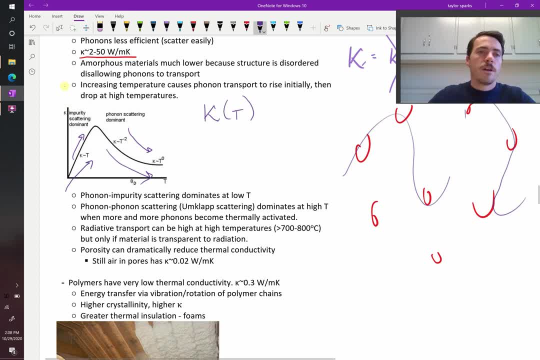 then you made it worse, right, Because now they scatter off one another. That said, you reach this minimum value. Most materials exhibit a minimum thermal conductivity. It's not like it goes all the way to zero, right? That doesn't happen. It reaches a minimum value. 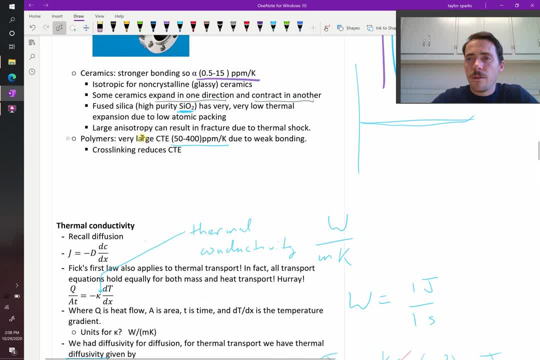 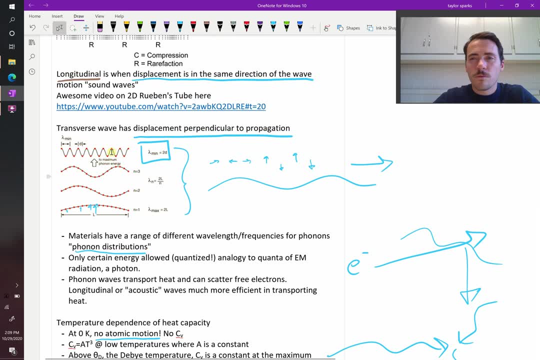 And that's because, if we remember, our phonon vibrations have a minimum wavelength that they can have. way down here, Our average interatomic distance is the smallest wavelength that we can have, So you can't scatter waves any more than that Once they're basically being 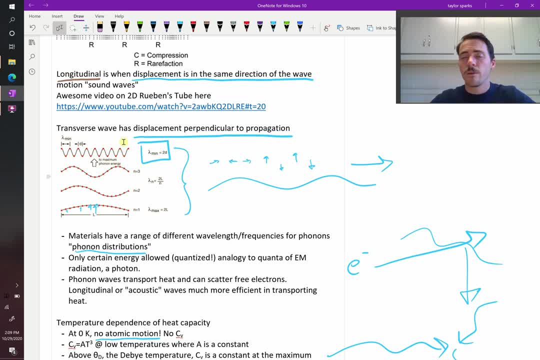 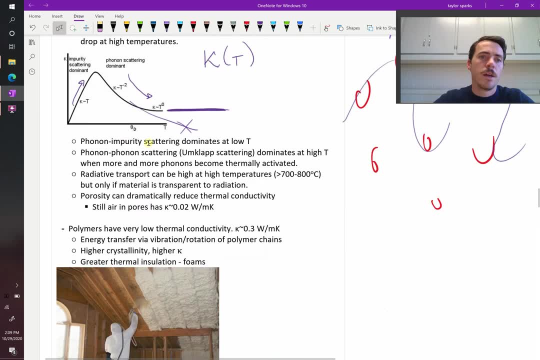 scattered at the atomic wavelength they can't be scattered anymore. So that puts a hard limit for most materials on the minimum thermal conductivity that you can have for these ceramics. okay, So we call this phonon impurity scattering at low temperatures. Any phonon that. 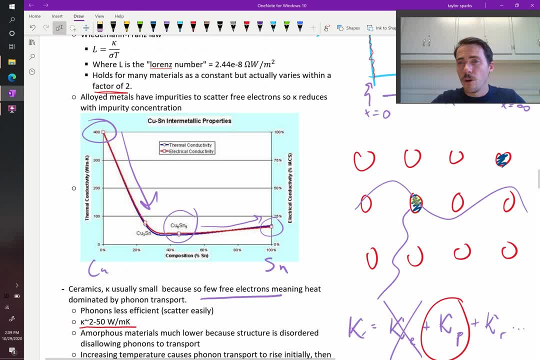 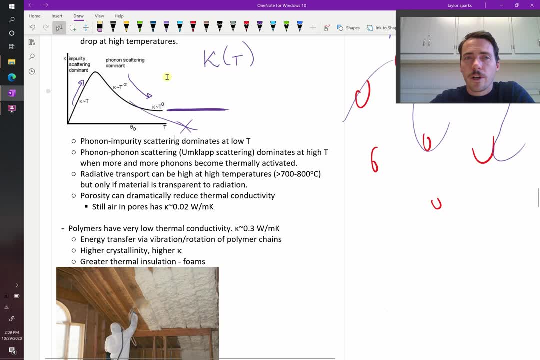 gets scattered is probably getting scattered off of like impurities in the lattice, like dopants, right, But at high temperatures we call this umklop scattering. That's when phonons scatter off of one another. One vibration hits another one and they it messes up there. 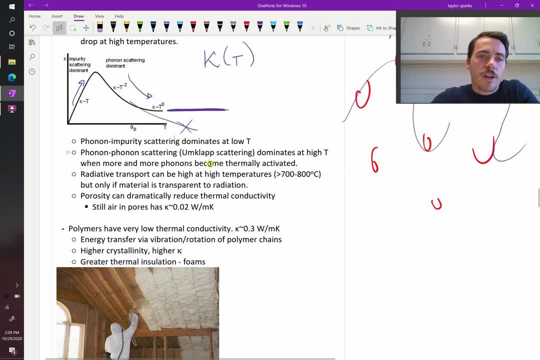 traveling through the material. okay, Radiative transport can be significant, but typically it's a high temperature process. It goes. the Stefan Boltzmann law says that you get, you know flux. it's proportional to temperature, to the fourth, I think. So it really takes off at high temperatures. 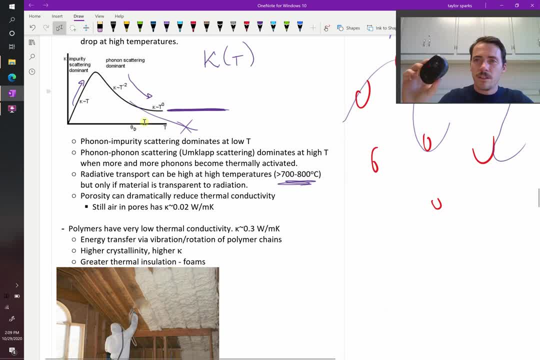 and it can be minimal. Like my mouse, it's not that hot. It technically is giving heat off, but it's not like I feel it like as if this was white hot. If it's white hot, you can really feel it coming off, because it's at high temperatures, right, So the flux greatly increases, okay. 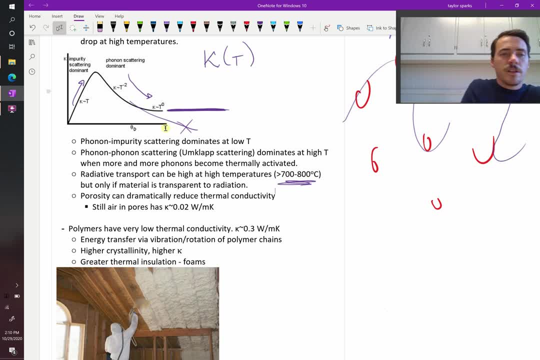 And things that you can do to change thermal conductivity ceramics is that you can introduce pores in them. We've already talked a fair bit about why ceramics have pores. Remember, a bunch of these particles have to sort of shrink together and once they solidify, you get rid of. 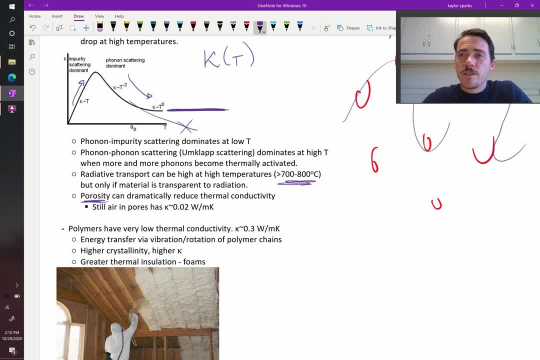 those pores. Well, if you don't get rid of those pores, if there's porosity left over, then you can end up with a really efficient way to reduce your thermal conductivity. because air pockets, particularly small air pockets, where they don't have convection, meaning the air is not flowing around in response to density- 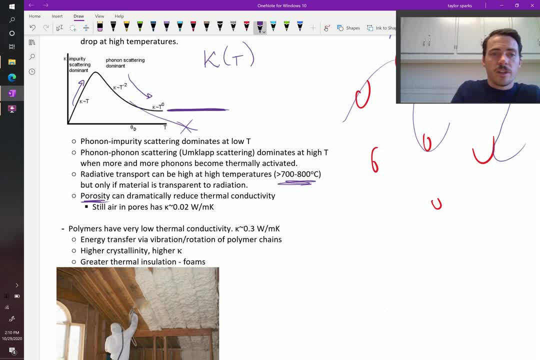 gradients. that has really low thermal conductivity. Still air, meaning small air, pockets. its thermal conductivity is 0.02 watts per meter Kelvin. So what's that? A hundred times lower than even low thermal conductivity ceramics. So that is, for example, why, when they make windows, 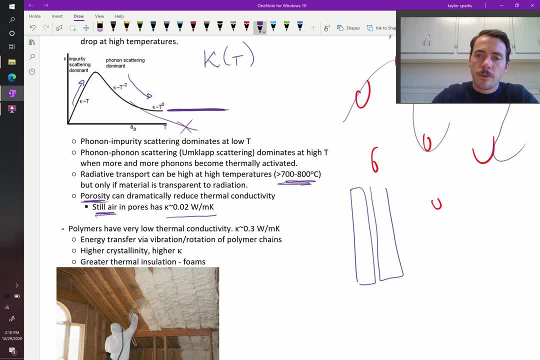 when they make windows they want to make that gap really small, but they put a gap. a dual-paned window has glass right here. it has glass right here, and then it has a little air gap right, The air gap in the middle. 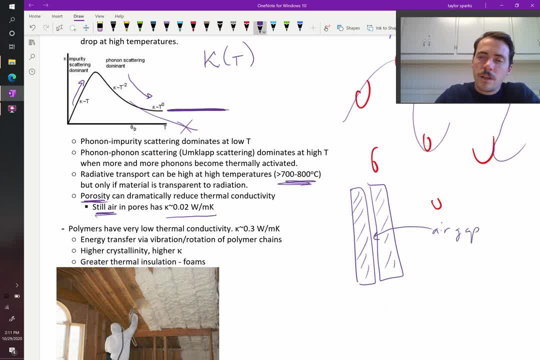 is because that is the worst conductor of heat than the solids, right, Which makes sense, because it's not a solid, so phonons are not going to travel through it very well, right, It's going to have, it's not going to have phonon transport. So again, if we go back up to our equation, 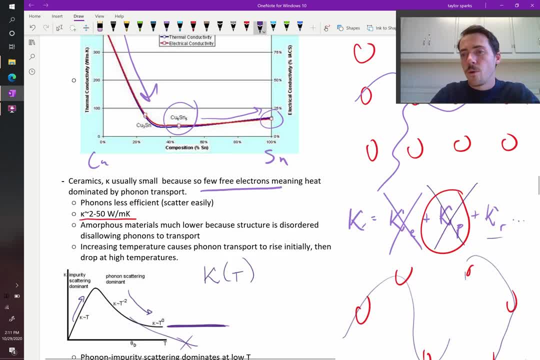 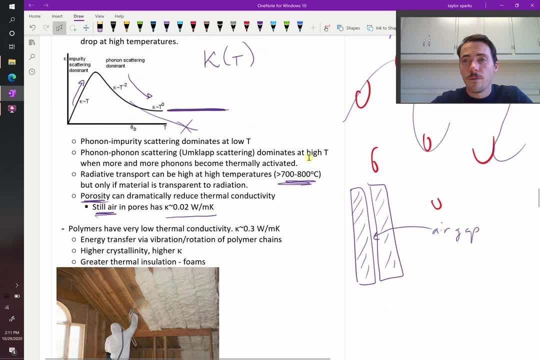 if you drop out phonon transport then you have to rely on radiative or convection. So now convection is what dominates thermal conductivity in air, especially still air. Then you get rid of that even you just get radiative. Okay. 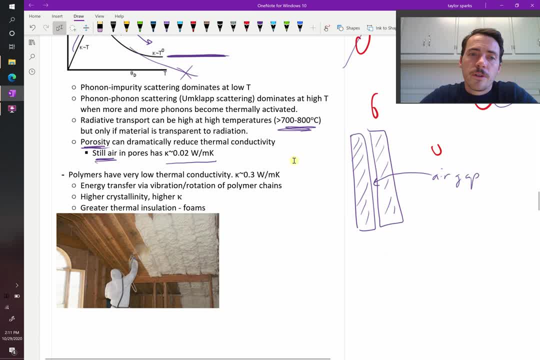 let's finally talk about polymers. Thermal conductivity of polymers is typically very, very low. You can get values of like 0.3 watts per meter Kelvin. So it's still 10 times greater than foam. right Air air pockets in foam, but it's 10 times less than most ceramics. 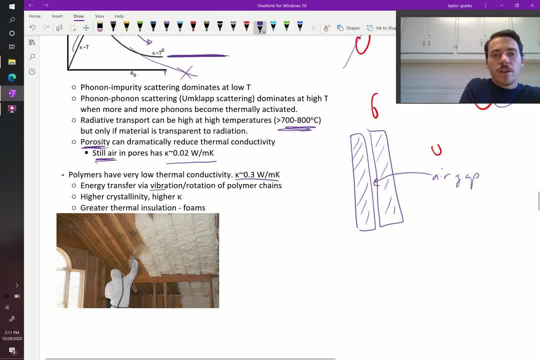 Where does the energy transfer come from? It comes from vibration and rotation of these polymer chains, right. So as a whole chain now can vibrate, it could technically conduct heat, but that's not nearly as efficient as individual atoms being able to form vibrations, right. 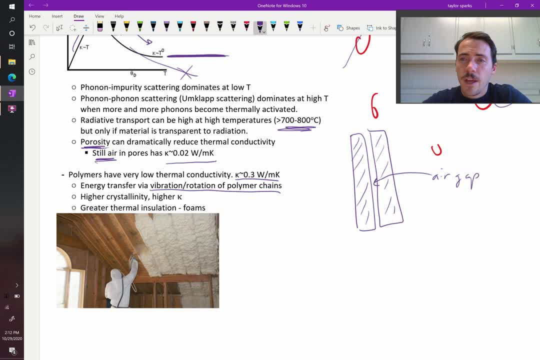 Obviously you can make polymers that are more crystalline and less crystalline and as you increase the crystallinity you're going to make it better for vibrations to travel through it, So you get higher thermal conductivity for high crystallinity polymers like PET or Kevlar, things like that.